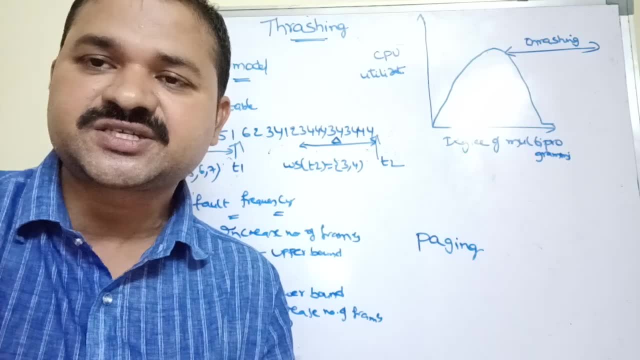 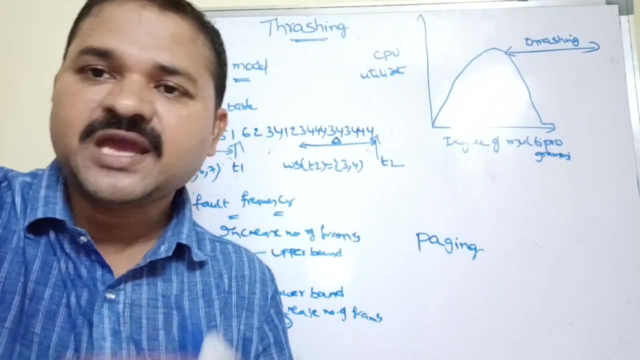 memory. So page fault occurs. So whenever a page fault occurs then operating system has to load that page from secondary memory to the main memory. So, but before that the page in the main memory will be transferred to the secondary memory. So that process is known as paging. So 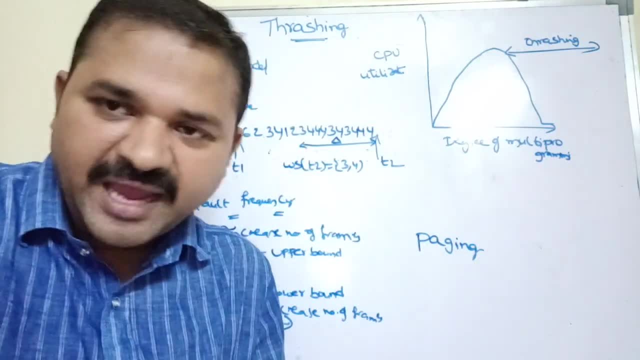 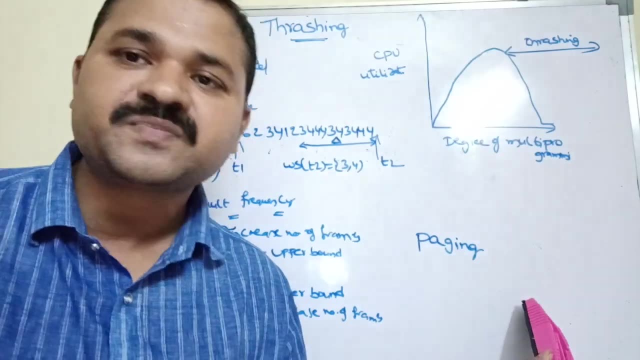 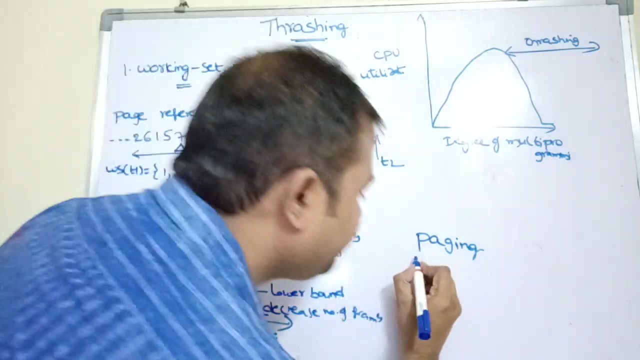 paging means swapping the pages between main memory and the secondary memory. So the definition for trashing is: if a process spends more time on paging rather than executing, then it is known as trashing. So let's see when the trashing will occur. Let me have a process: process people. 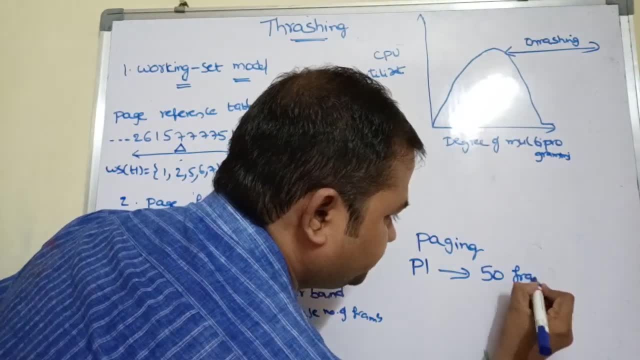 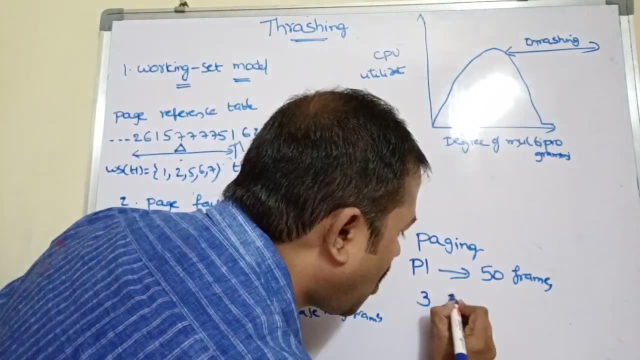 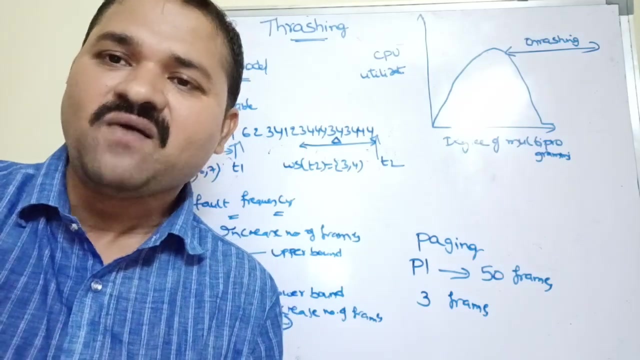 Let, process P1 requires 50 frames. So totally 50 frames are required for executing process P1. Whereas let us assume that operating system allocated only 3 frames to process P1. So that means here process P1 doesn't have enough number of frames for its execution. So what will happen? 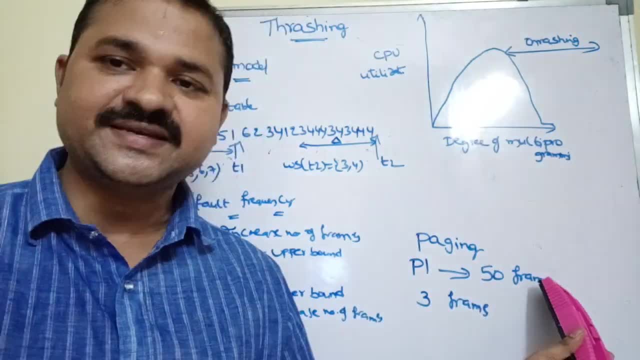 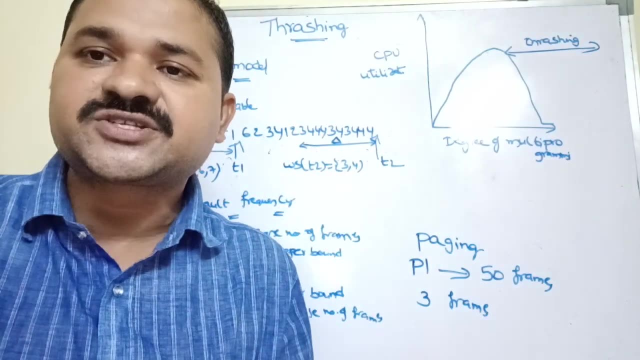 Too many page faults will occur. Why? Because here we have 50 pages whereas only 3 frames are allocated, So too many page faults will occur. So let's assume that operating system allocates only 3 frames to process P1. So if too many page faults occurs, then what will happen? We have 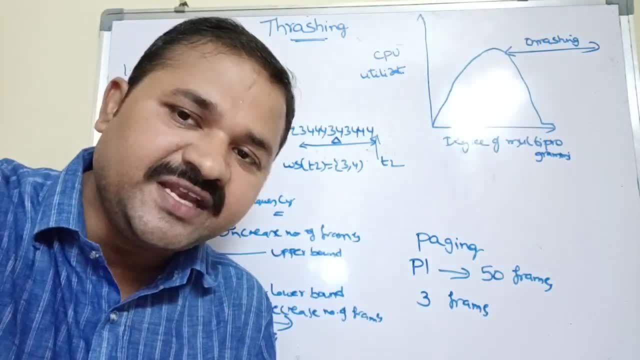 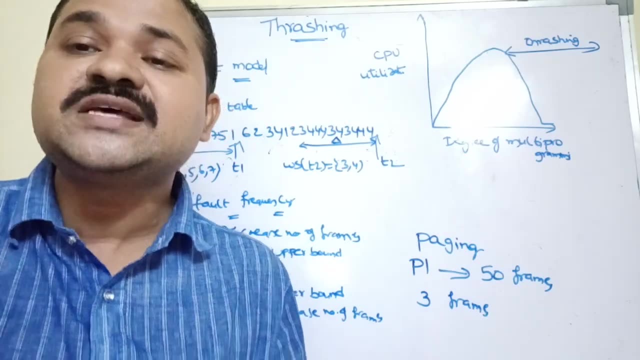 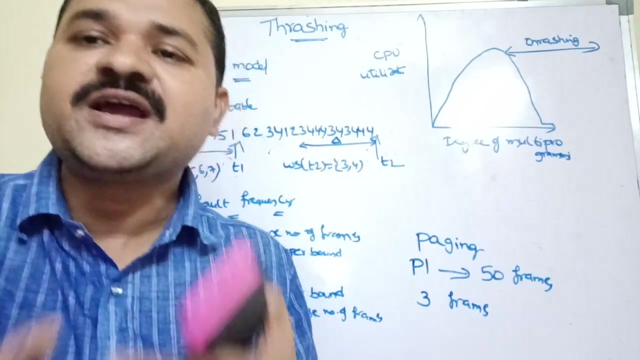 to transfer, we have to swap the corresponding pages between the main memory and the secondary memory, So the CPU utilization will become less. Why? Because here the process is spending more time on paging, swapping rather than executing, So CPU utilization will become less. So what? 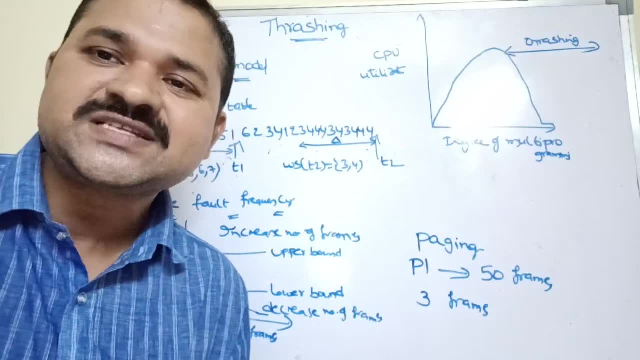 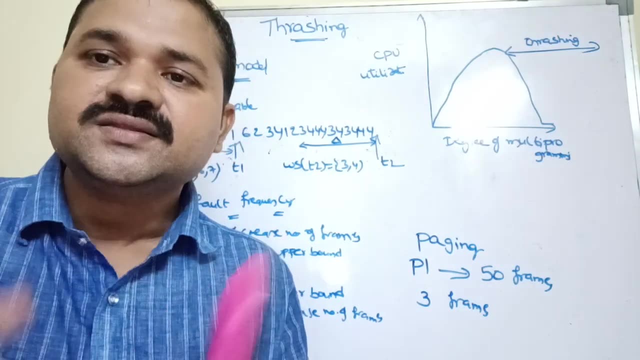 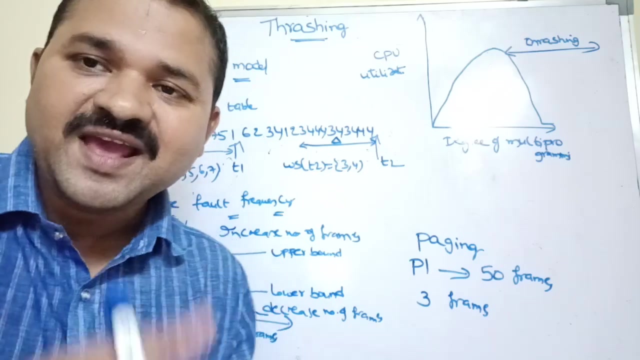 the operating system will think is main memory contains only limited number of processes, So that's why CPU utilization is low. So, in order to utilize the CPU in an effective manner, operating system replaces more number of processes in the main memory. So what will happen now? So, 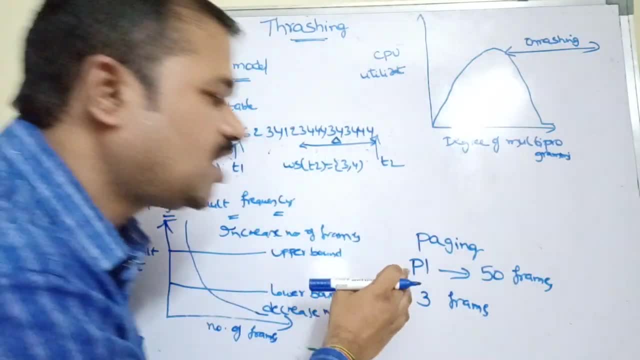 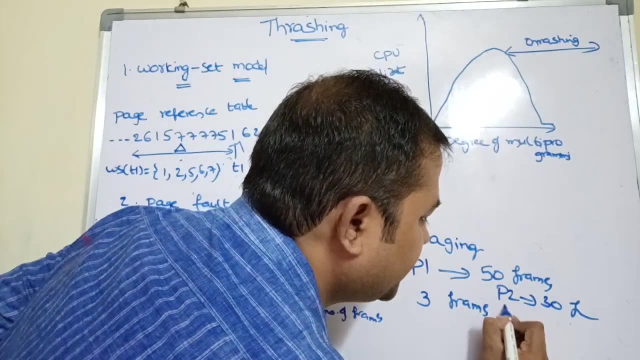 let us assume that two more processes are placed in the main memory. Let the demand for those processes is: let: process P2 requires 30 frames, whereas process P3 requires some 20 frames. So what is the demand of P1, P2, P3?? So 50 plus 30 plus. 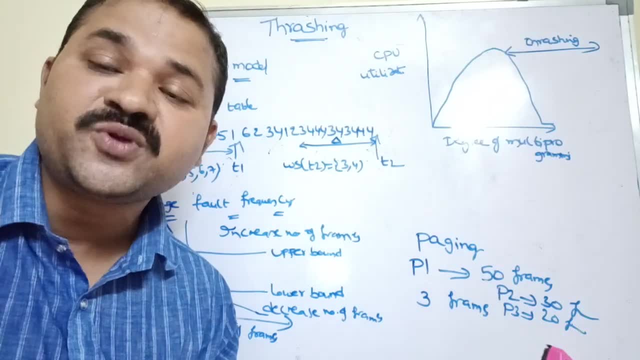 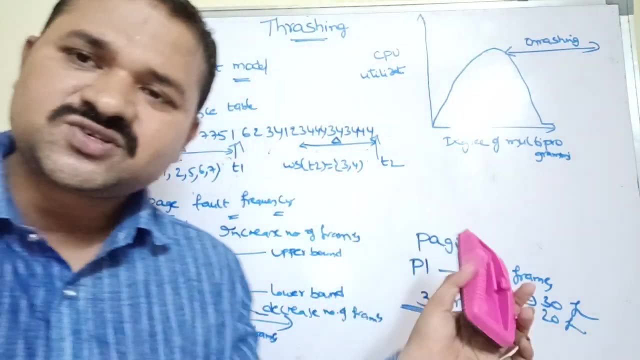 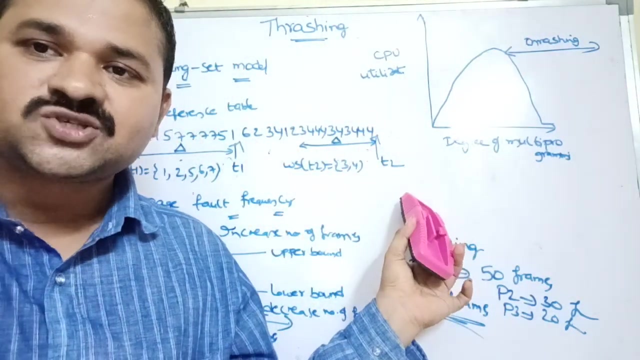 So 100 frames are needed for executing process P1, process P2 and process P3. Whereas operating system allocated how many frames? Only 3 frames. So what will happen? The page faults will become more and more and more So. this situation is known as trashing. So here what is the 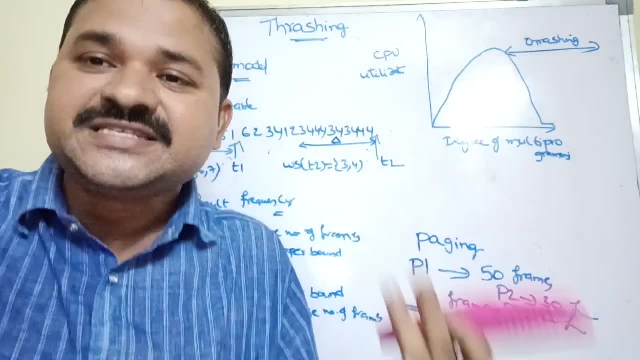 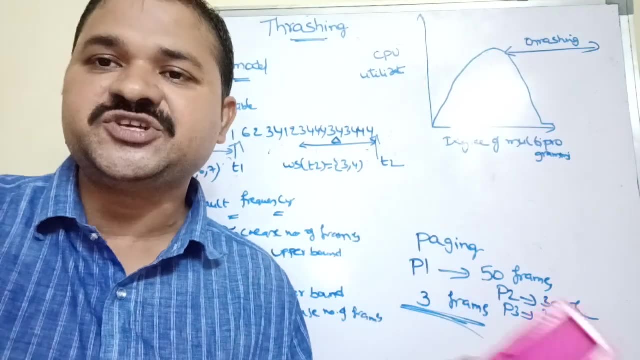 problem here. The process is spending more time on paging rather than executing, So this is known as trashing. So we can avoid the trashing, We can handle the trashing. So we can handle the trashing using two techniques. First one is working set model. Second one is: 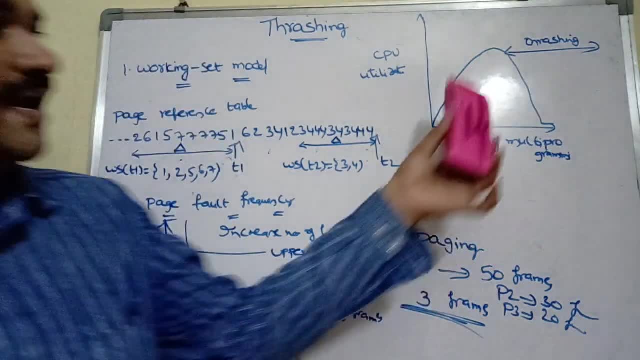 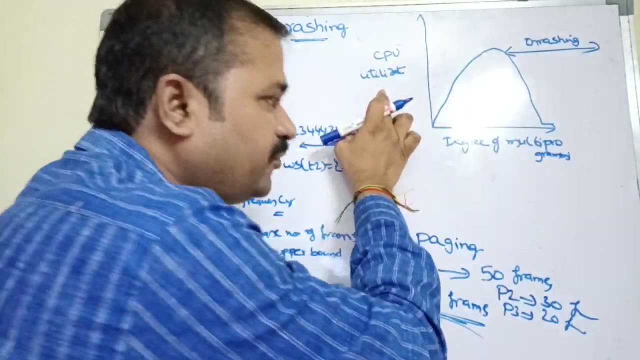 page fault frequency. So before discussing these techniques, let us see the diagram for trashing Here: x-axis represents degree of multiprogramming, Y-axis represents CPU utilization. So we know what is degree of multiprogramming. So degree of multiprogramming means placing more number of 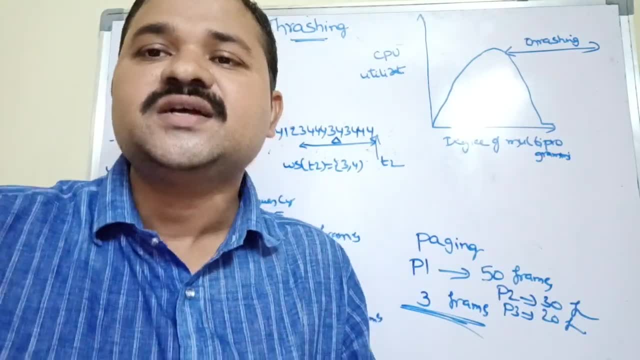 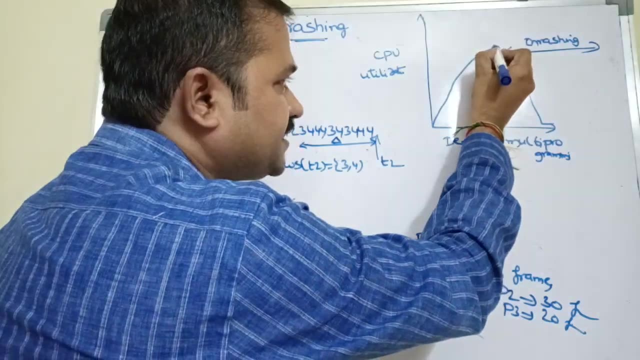 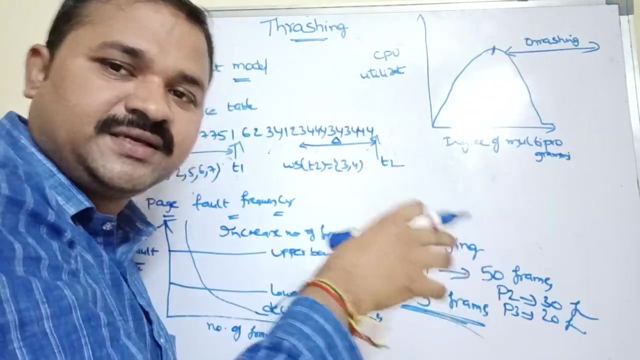 processes in the main memory in order to utilize CPU performance in an effective manner. So this is y-axis represents, Then c-axis represents CPU utilization. So up to this point CPU utilization is excellent. But after that, let us assume that operating system places more number of processes in. 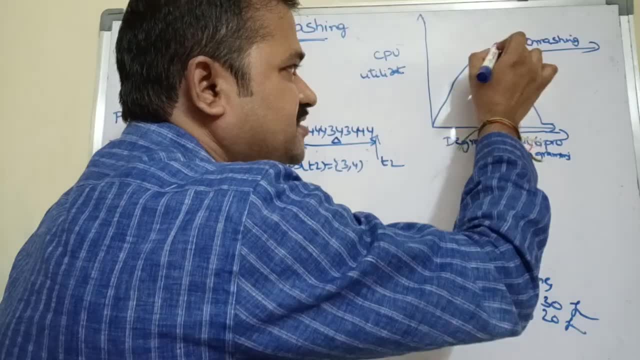 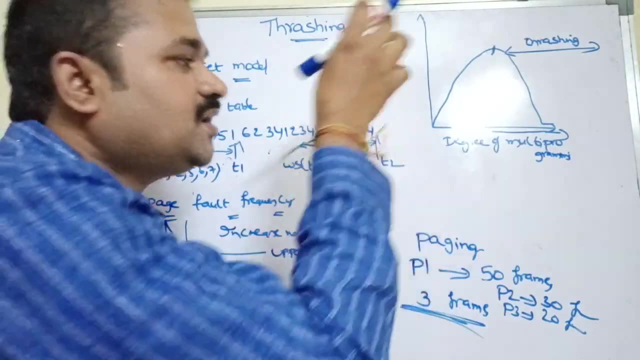 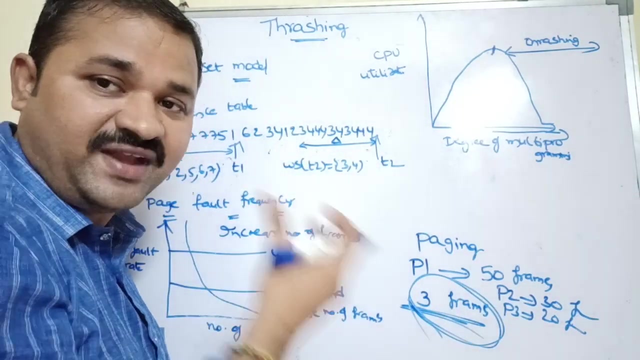 the main memory. So this is nothing but x-axis. After that, what was happened? Let us assume that operating system places more number of processes in the main memory, So for those processes, only less number of processes- Exactly number of frames- were allocated. so what will happen now? paste files will become more so. whenever paste files become more, then swapping will be needed between the primary memory and the secondary memory. so what will happen? cpu realization will comes drastically down. why it comes drastically down? why? because here the process is not spending time on executing, it is spending more time on the swapping the pages between primary memory and the secondary memory. 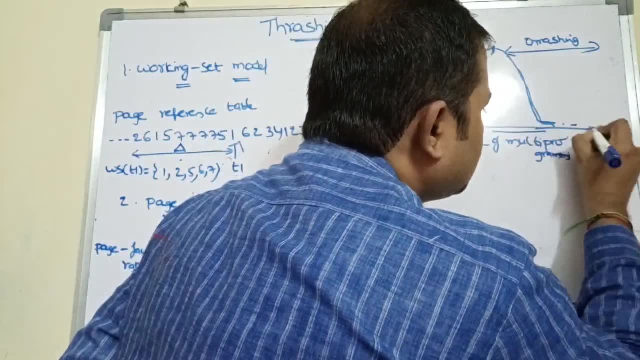 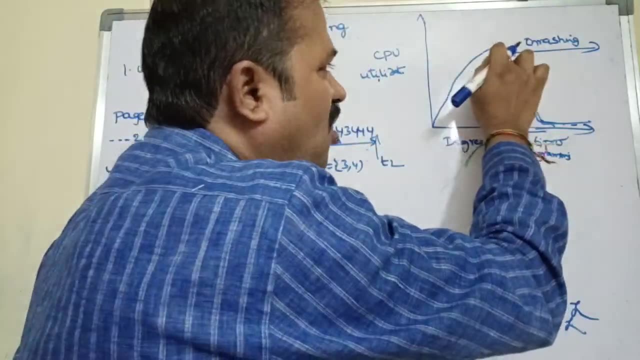 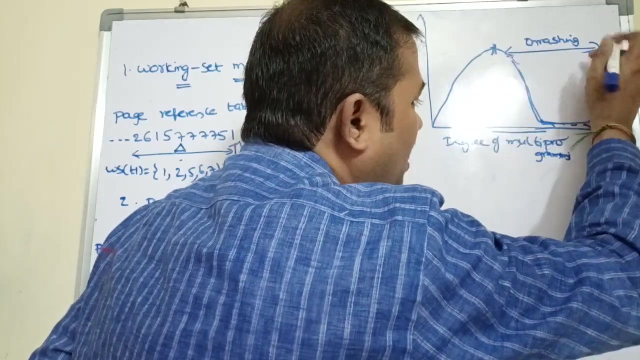 so this, this portion, so this portion is known as trashing. so up to this point the cpu utilization is excellent. but after that cpu utilization falls down drastically. so this situation, this drastically fall down, is known as trashing. so whenever a trashing occurs, then operating system. 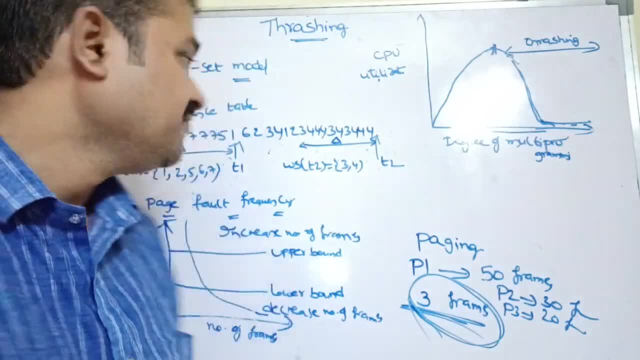 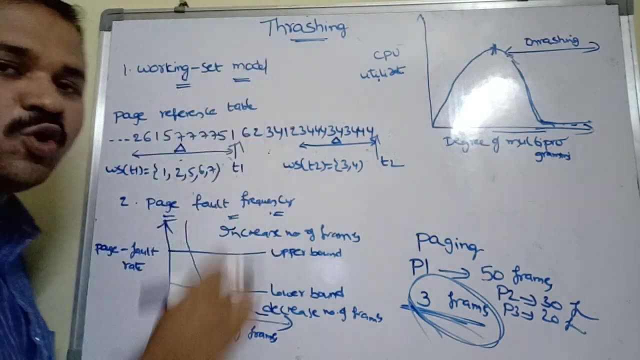 will not work. so whenever a trashing occurs, then operating system will not work. so whenever a has to handle the trashing. in order to handle the trashing, we have two approaches. the first approach is working set model. the second approach is pays for frequency. let's see about works, working set. 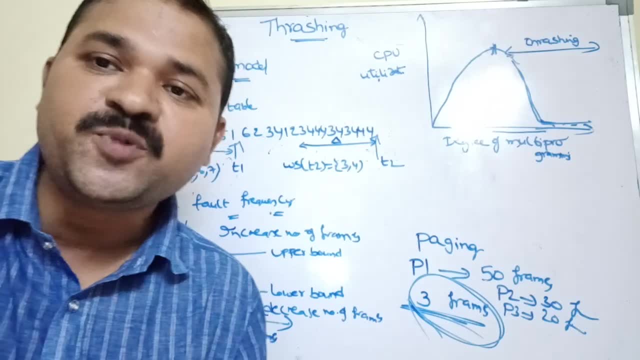 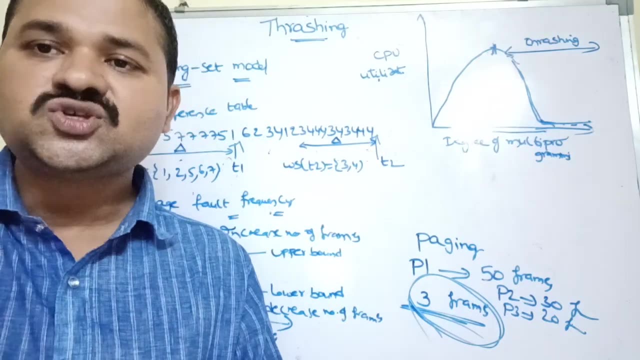 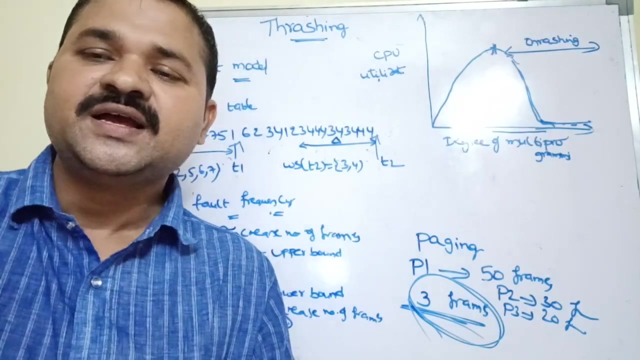 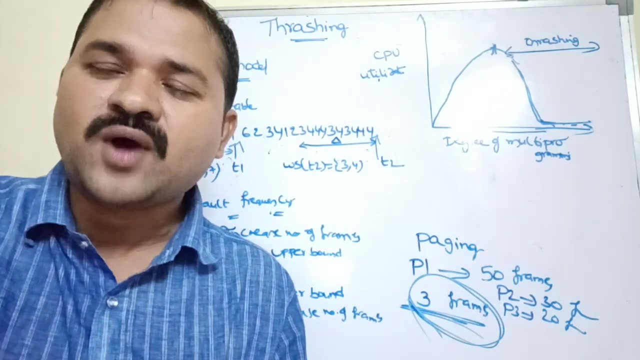 model working, set model works based on the principle of locality of reference or principle of locality or locality model. so we know what is locality of reference. locality of reference specifies that over a short period of time, a certain information or executive repeatedly and repeatedly, if you take a far loop, for is equal to zero, i less. 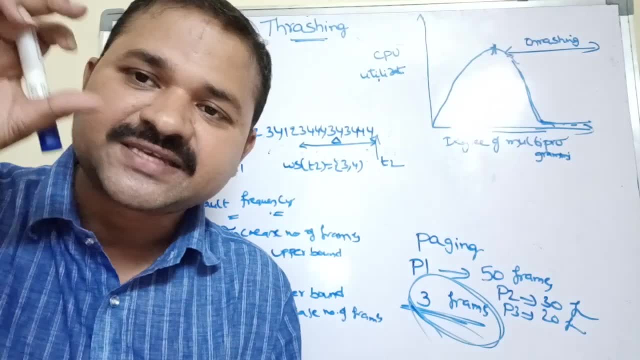 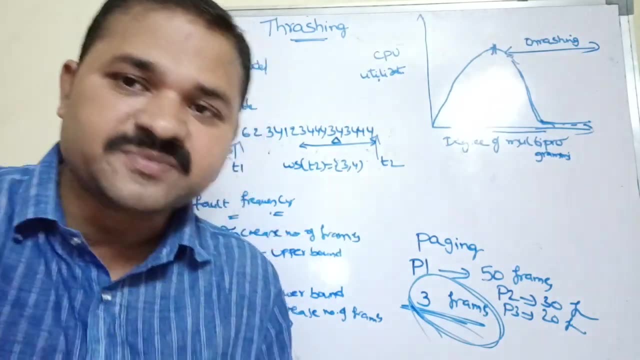 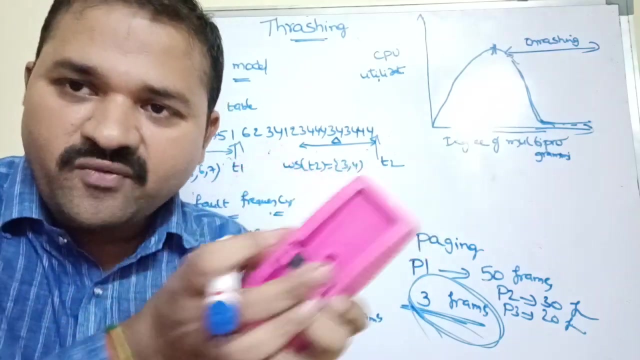 than hundred, i plus plus. let us assume that parloop contains five statements. so how many times those five statements will be executed? those five statements will be executed hundred times. so that means we are executing those statements repeatedly. so that is nothing but locality of reference. so over a short period of time, a certain number of instructions are executed repeatedly, and 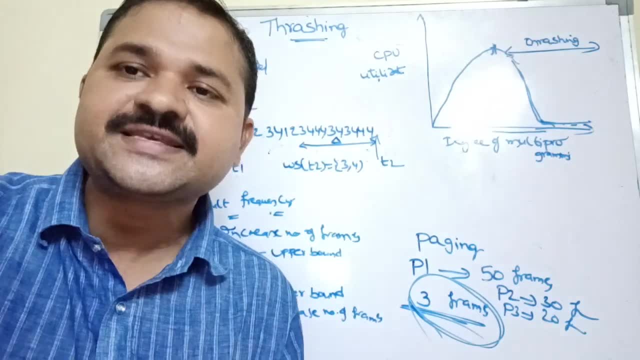 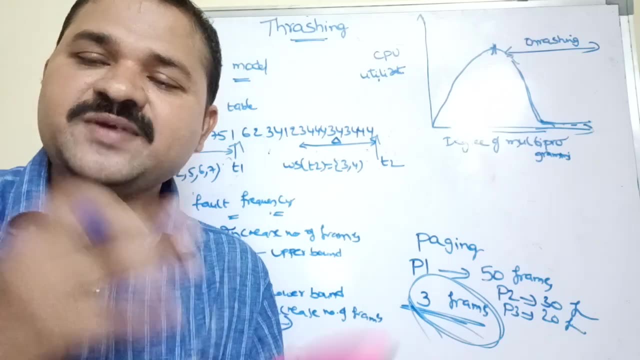 repeatedly and that specific information can be executed always. these people haven't written a. If you take a C program, a C program is a collection of functions. So let me call a function 10 times. So what will happen? The statements within the function will be executed 10 times. 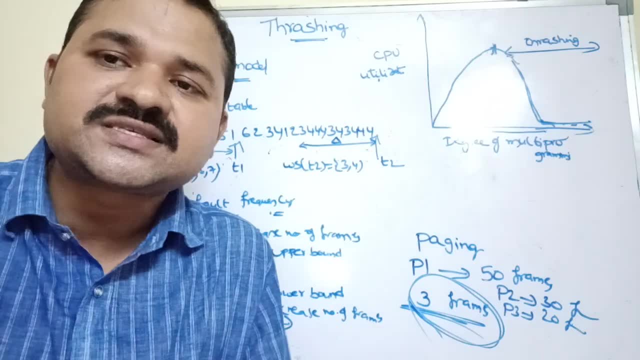 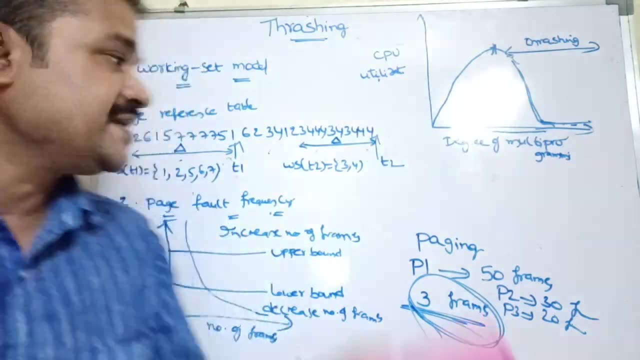 Why? Because we call that function 10 times, So as the process execution continues, then we move from one locality to the another locality. So here the point. here is the working set model works based on the principle of locality, of difference. 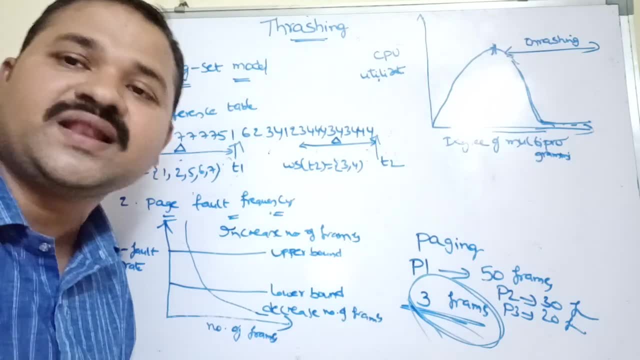 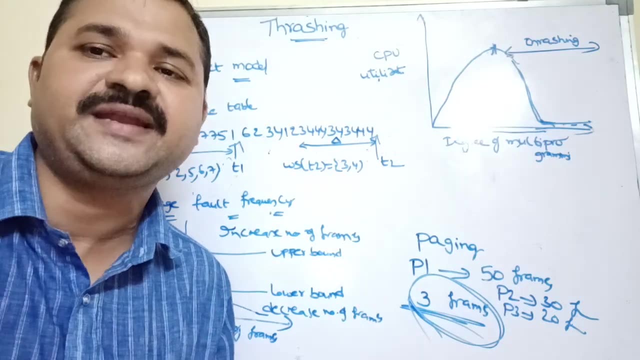 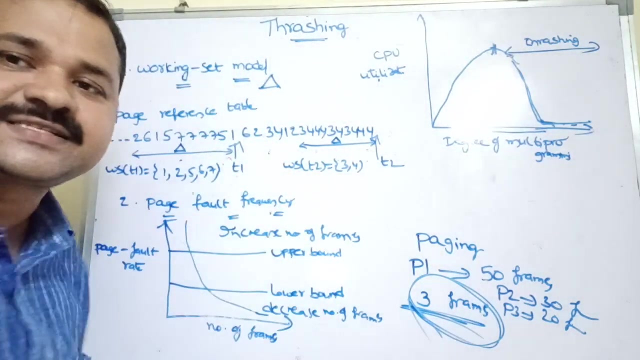 So locality of difference or principle of locality or locality of model. So it specifies that over a short period of time a certain number of instructions are executed repeatedly and repeatedly. Here working set model is represented with the help of delta. Here working set model. it contains the set of active pages. 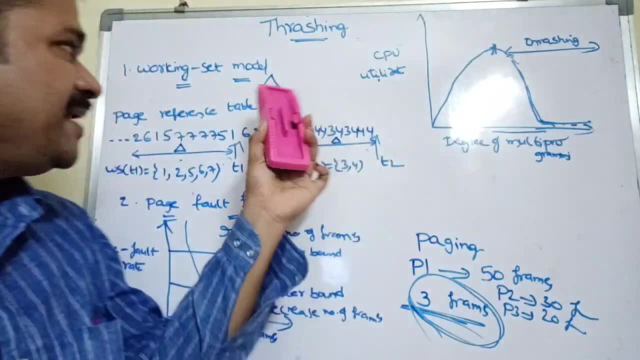 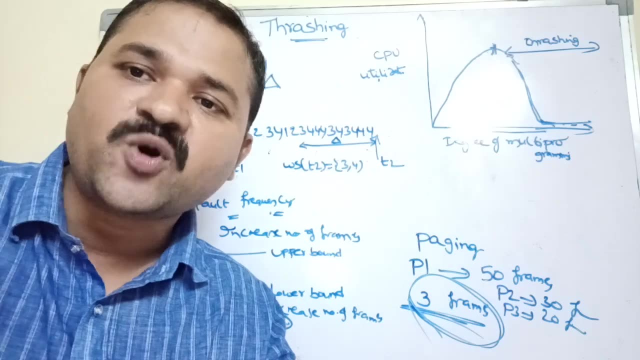 So if the page is active, then the corresponding page will be placed in working set, Whereas if the page is not active, then we have to remove the page from The corresponding working set. So we can represent working set with the help of a symbol called delta. 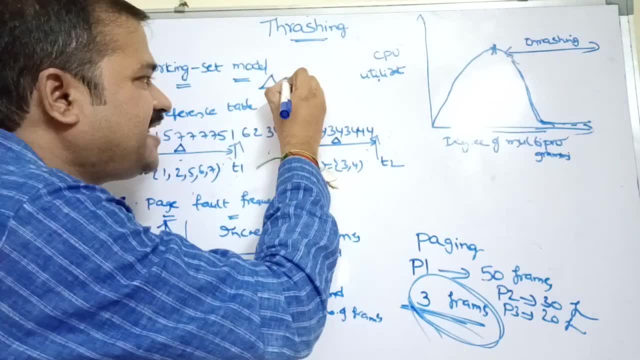 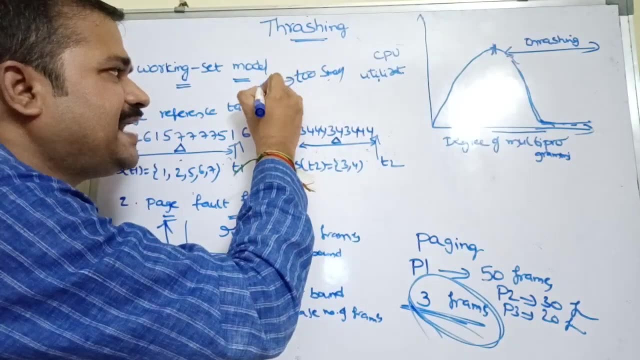 So how to specify the size for the delta. Suppose if delta value is too small, then the problem here is: if delta value is too small. So what is delta? here? Delta means the size of the working set. So what is working set? 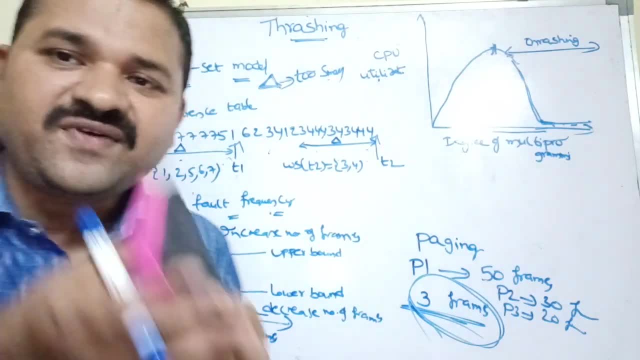 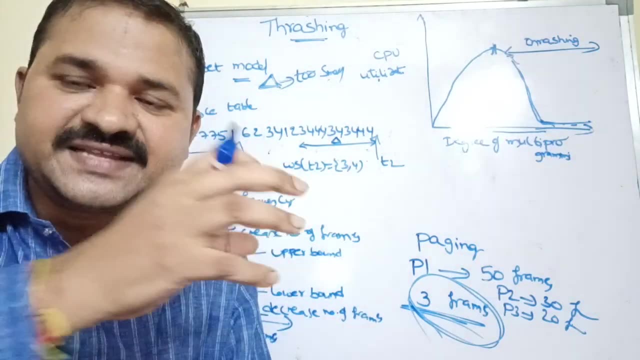 It specifies the set of active pages. So that means it specifies localities. So if you take a function, the first function is nothing but 1. So that is nothing but 1 working set. The second function will become second locality. 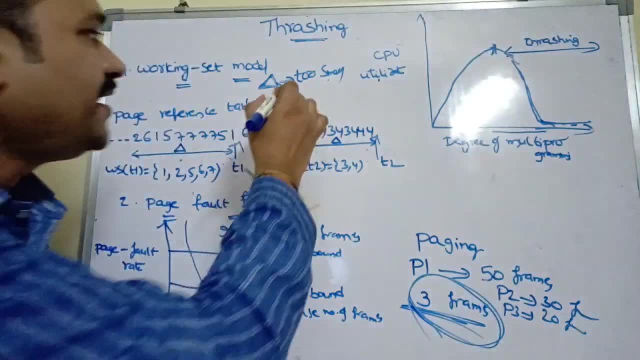 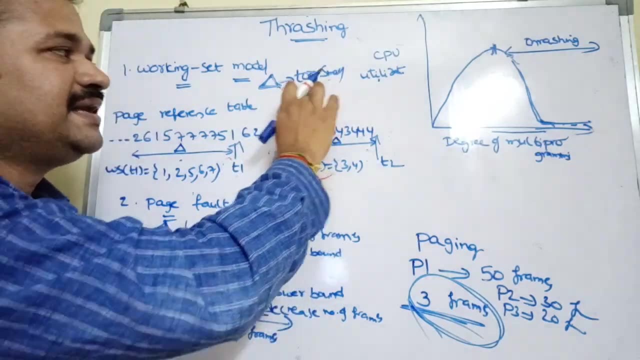 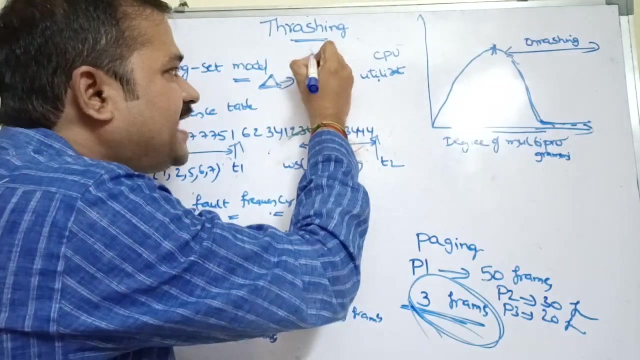 So that is nothing but second working set Like that. So here the point is how to select the size for the delta. Suppose: if delta value is too small, then it does not cover the entire locality. Let: in order to execute a function, we require 10 frames. 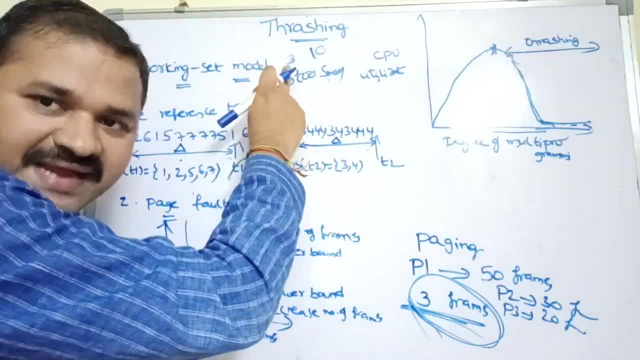 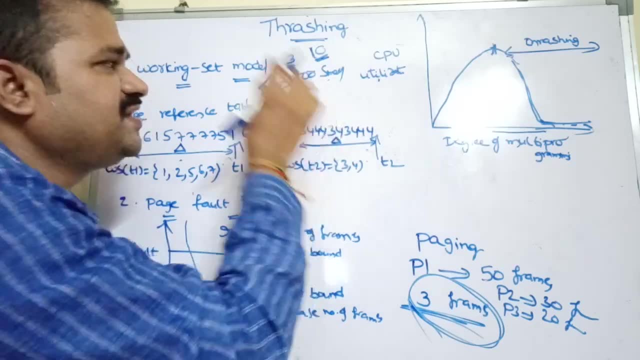 Whereas we allocated only 3 frames. So that is nothing but delta. So how many frames? We allocated here? 3 frames, So this is too small, Whereas what is the demand of the corresponding locality? 10 frames. 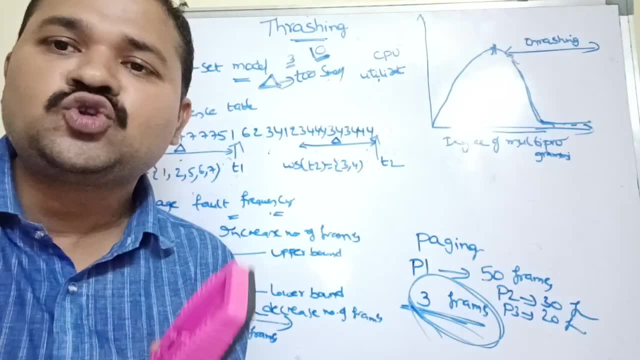 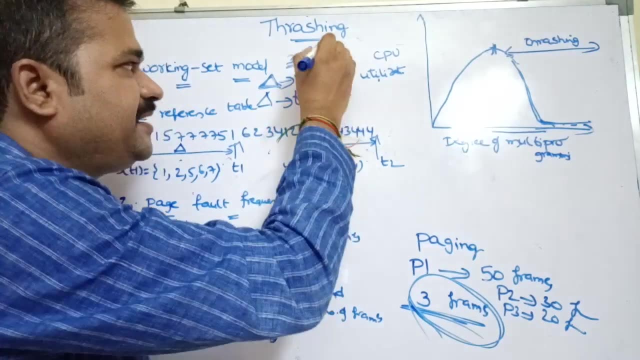 So what will happen? It does not cover the entire locality, So too many page falls will occur. And the second point is suppose, if delta is too large? So that means let us assume that here the demand is, the demand for that locality is 10 frames. 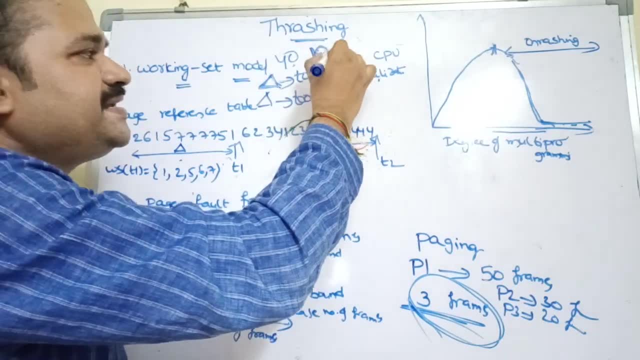 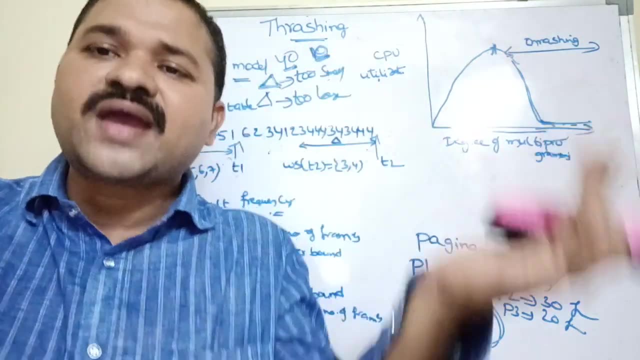 Whereas we allocated 40 frames. But what is the demand here? Only 10 frames, But how many frames? we allocated 40 frames. So what will happen? It covers the remaining localities also, So it stores the remaining functions pages also. 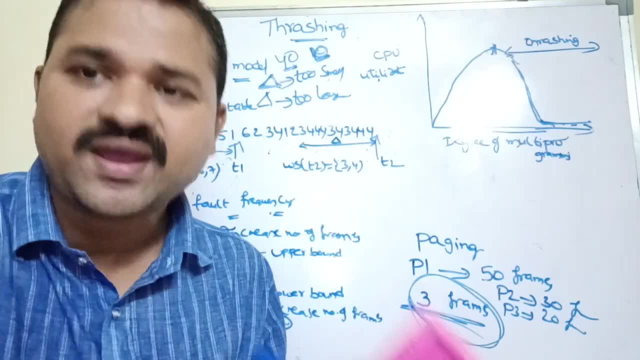 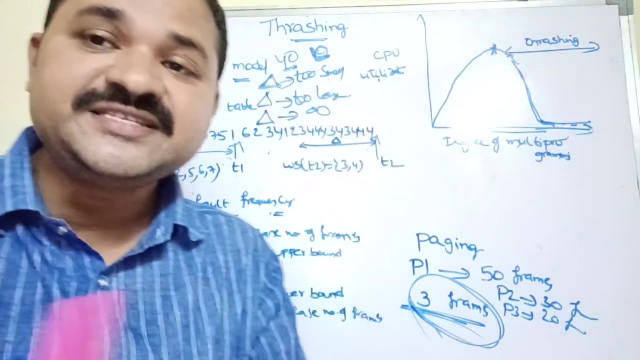 But that is not needed here. At a time we execute only one locality And the next criteria is delta value may be infinity. Suppose if delta value is infinity, then it can store the pages of the entire program, So it covers the entire program. 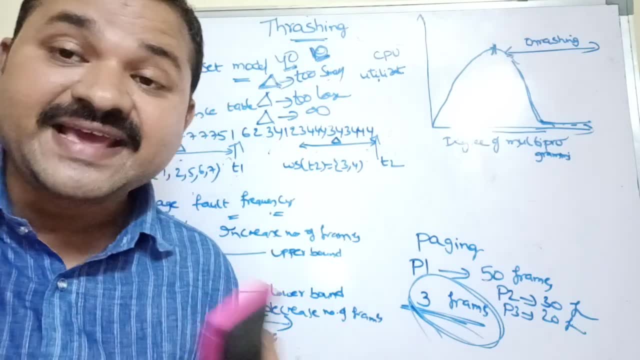 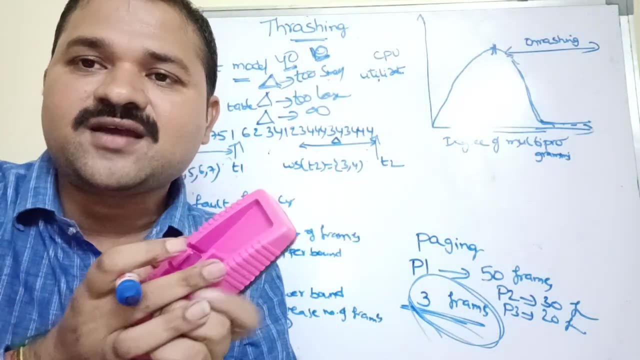 So that is about delta. So what is delta? It is a working set. So what is a working set? It contains a set of active pages. So we can say that we can take delta value as too small or too large or infinity. 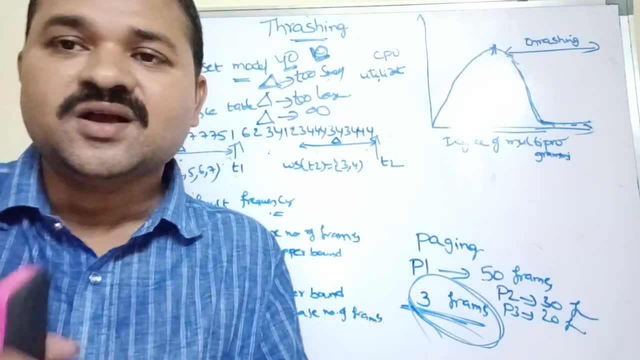 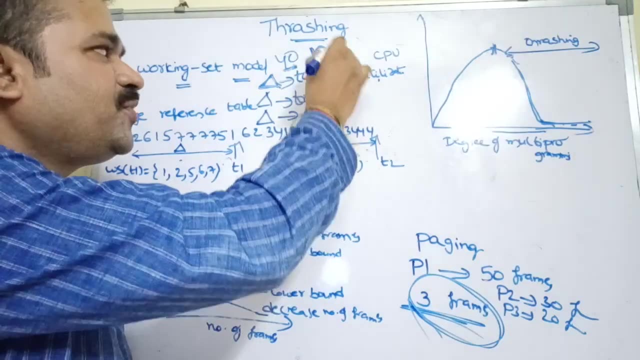 So if we take delta value as too small, then what is the problem here? More number of page falls will occur. Why? Because less number of frames are allocated to the corresponding process. So if we allocate less number of frames to the process, then the number of page falls will become increases. 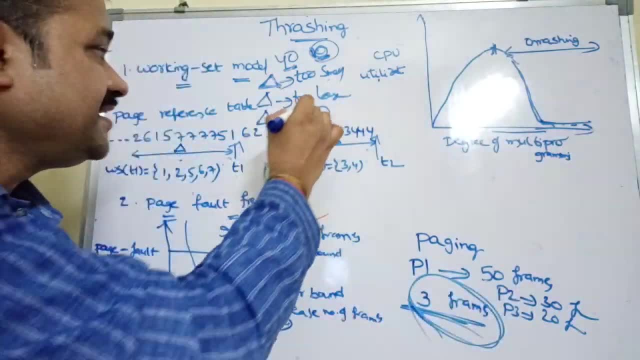 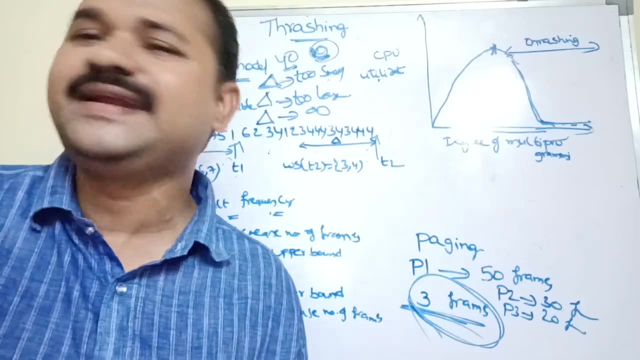 Suppose, if delta value is too large, Then what will happen? if it is too large, then it stores all the pages. then it stores all the pages of the program, but not- but it is not needed here at a time we have to execute that locality- pages only. 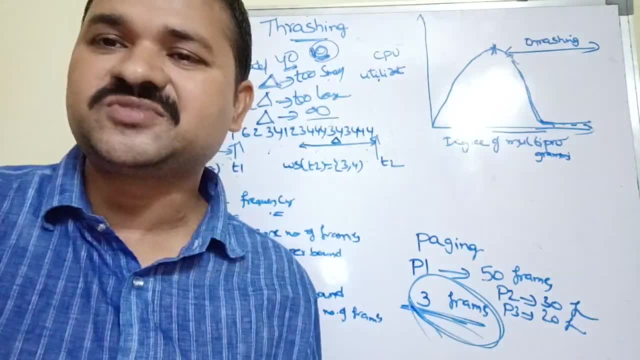 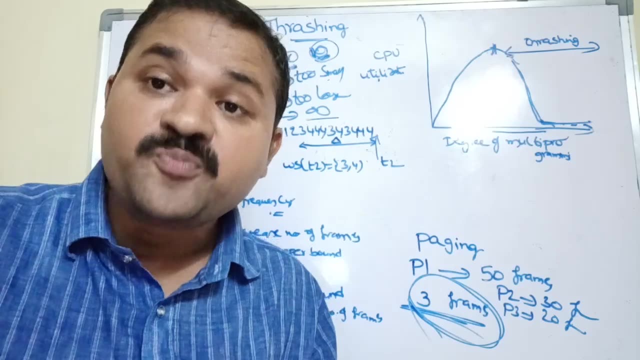 Next, if delta value is infinity, then it can store the entire program. So this is also not needed. So, depending upon the size of the locality, operating system has to allocate the number of pages for the corresponding locality. So for that, let us take this example. 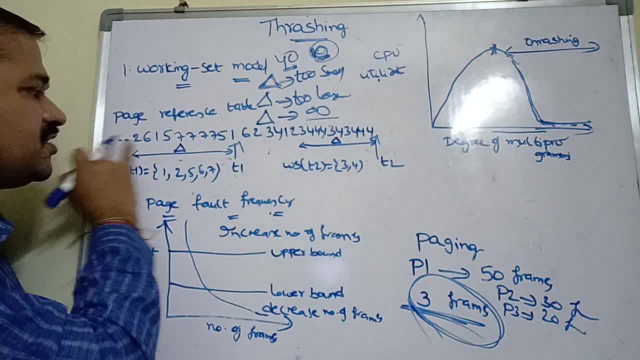 This. this is nothing but pages, So this is nothing but page reference table. So let CPU is executing these pages here. So first to second page, sixth page, one page, fifth page, seven, seven, seven, seven. 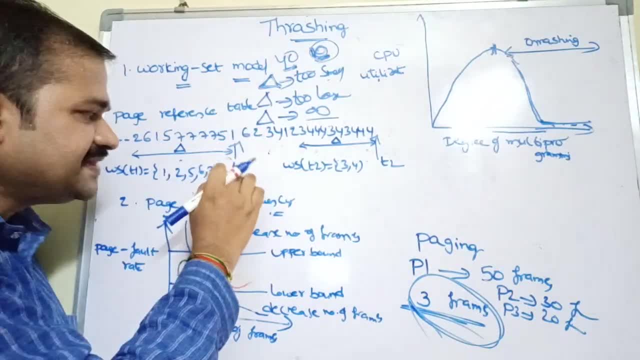 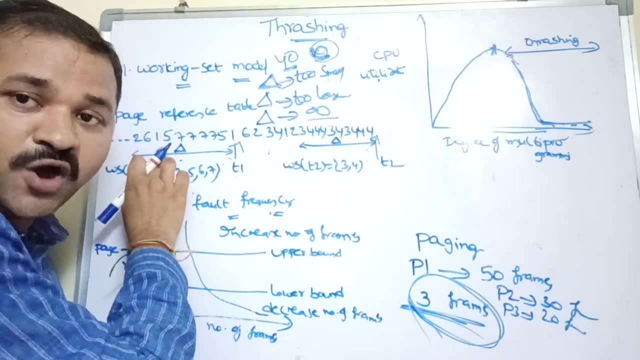 Likewise, we have several references here, So this is nothing but T1.. So at a time T1, the working set for the past ten references are. So how many page differences? we have taken Ten references, So this is nothing but one working set window. 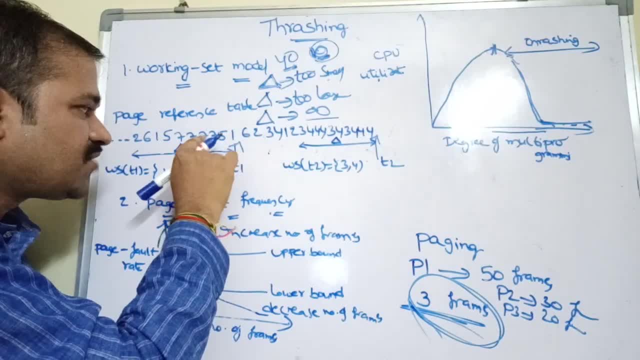 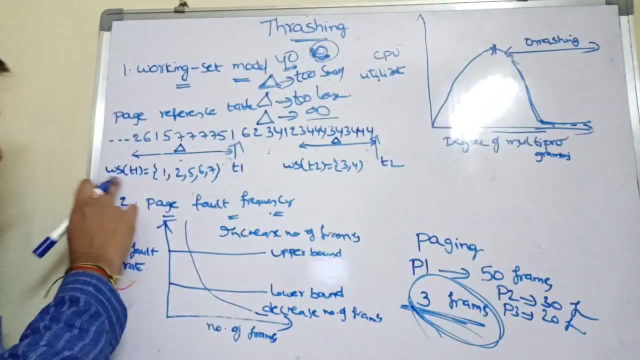 So ten references. This is nothing but first reference, Second, third, fourth, Five, six, seven, eight, nine, ten. So totally we have ten pages. So at time T1.. Then what is the working set window contains? 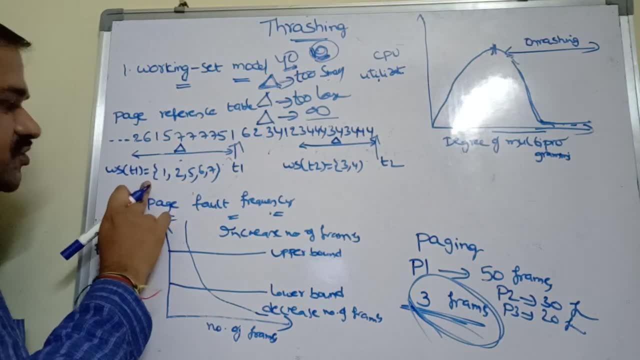 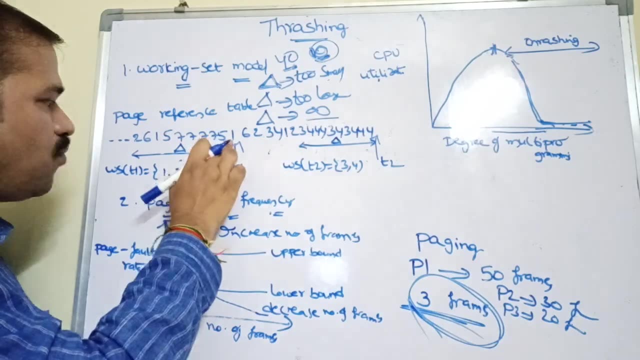 W is off. What is the time here? T1.. T1 is equal to. We know that working set always contains the active pages. So in the last ten references, what are the active pages? We have one, We have two. 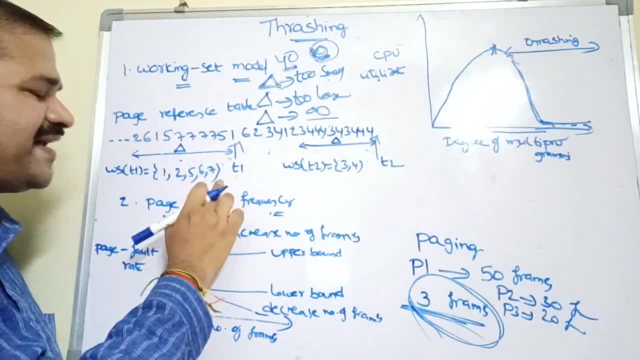 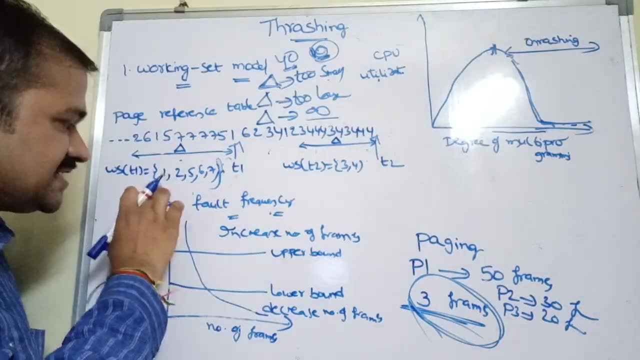 We have five, We have six And we have seven. So one, two, five, six, seven. So how many pages are there? Five pages. So now what the operating system will do is: Operating system allocates five frames for the corresponding locality. 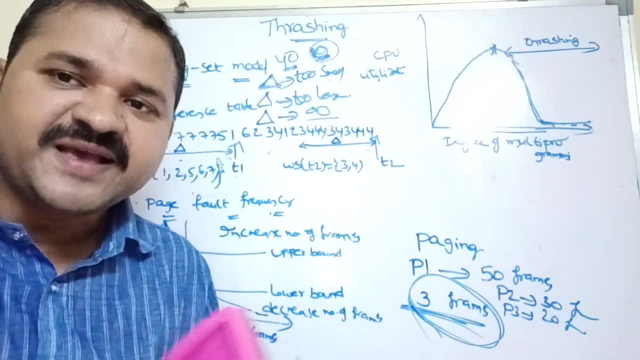 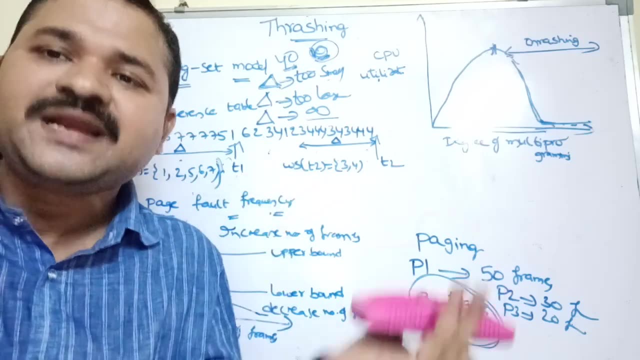 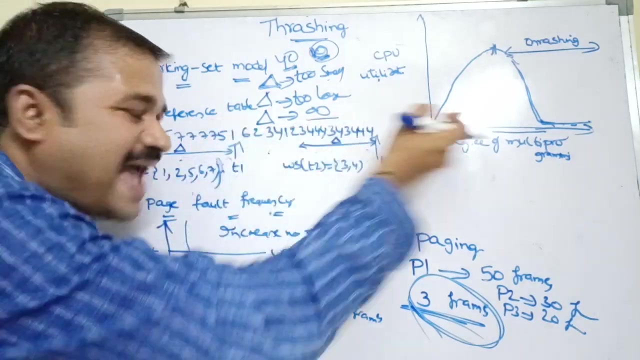 Why? Because here we know that working set model works based on the principle of locality of reference. So what is locality of reference? Executing the set of instructions repeatedly and repeatedly. So in the future also there is a chance that we may get one, two, five, six, seven pages very actively, very frequently. 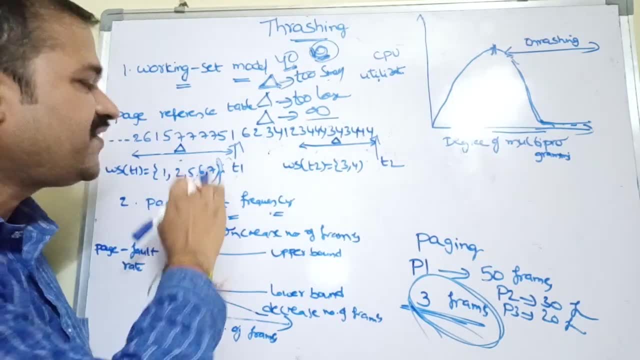 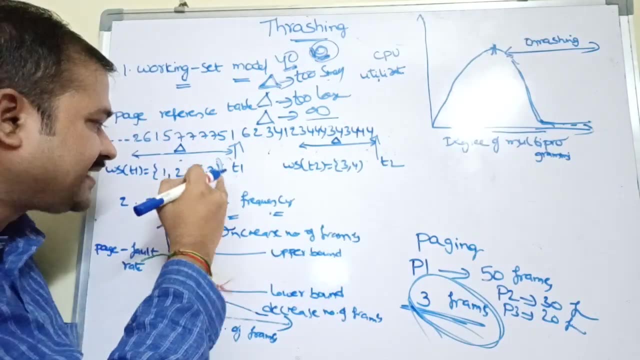 So that is why operating system allocates five pages for the corresponding For the corresponding process, So that in the future also there is a chance that we may get these pages very frequently. So there is no problem here, Okay. 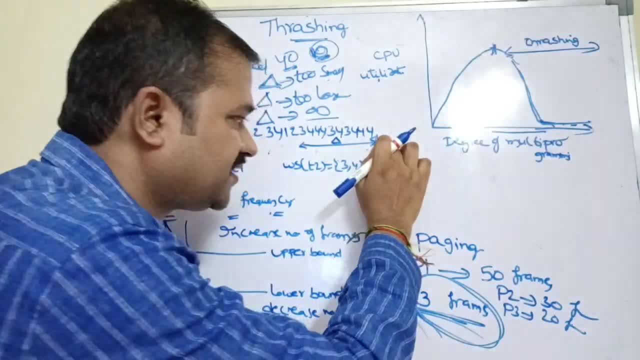 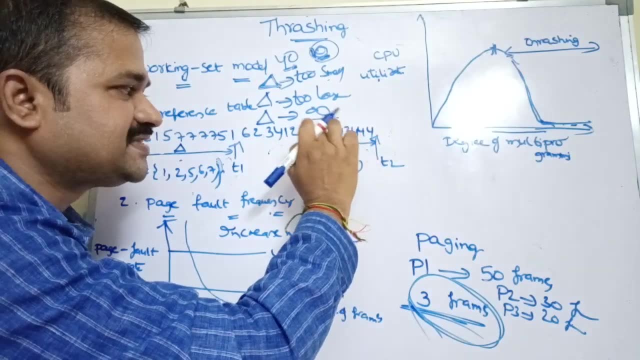 This is completely assumption based approach. Likewise, if you take this one At time, T2, for the past ten references, this is the working set window. So one, two, three, four, five, six, seven, eight, nine, ten. 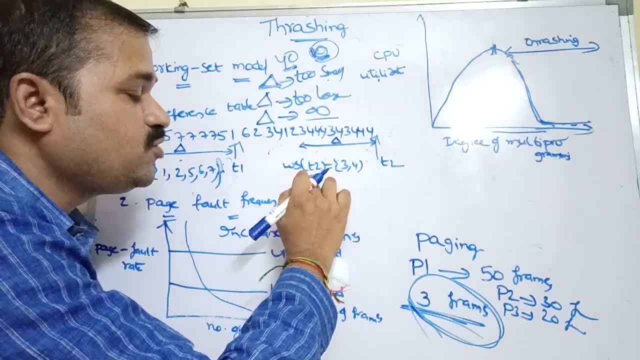 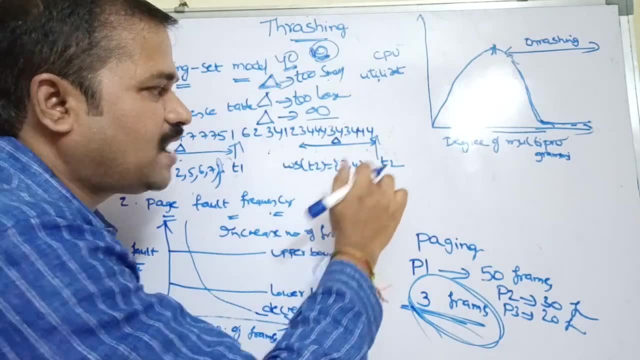 So what are the active pages here? in the past ten references, WS of T2 is equal to, So we have only two pages here active pages. First page is Three, second page is four, So three comma four. After that we may have some other pages. 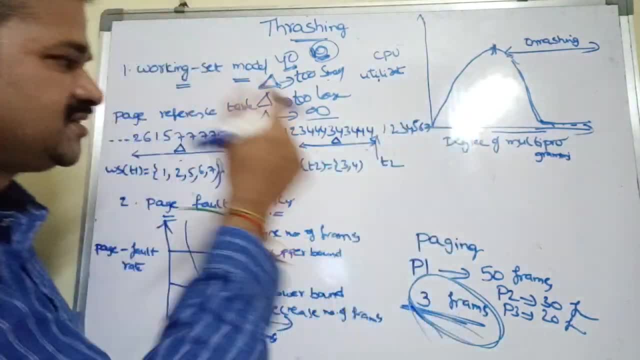 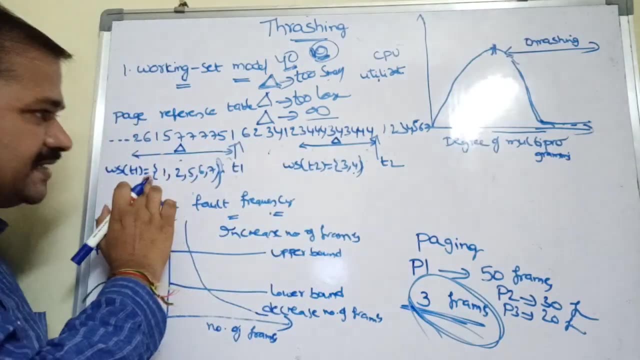 One, two, three, four. one, two, three, four, five, six, seven like that. So at time T2.. So what are the active pages here? Three, four, So that means here in these, in this working set window. these pages are not active here. 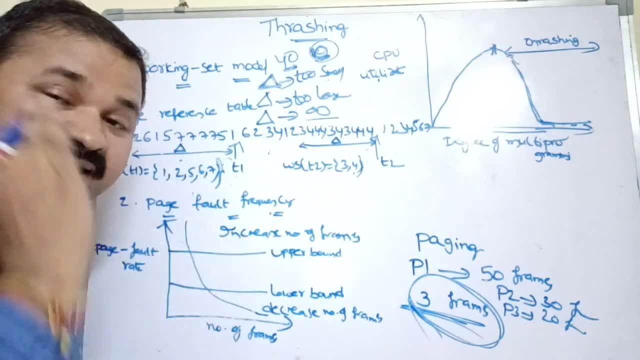 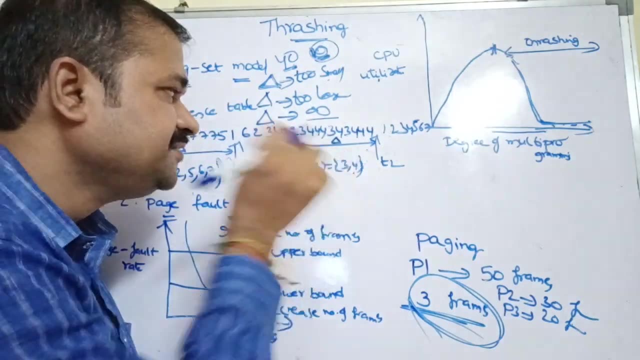 One, two, five, six, seven are not active, So that's why these pages are removed from the working set. And what are the active pages here? Three, four are the active pages, So how many frames need to be allocated for this locality? 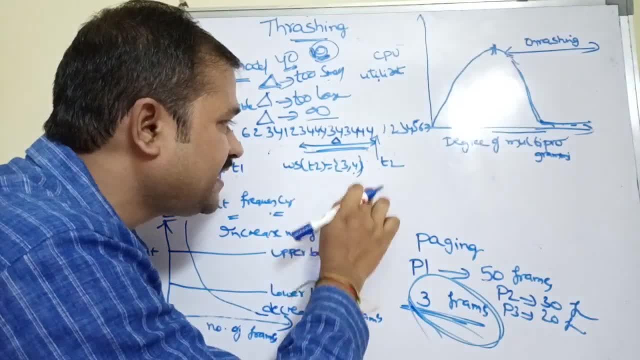 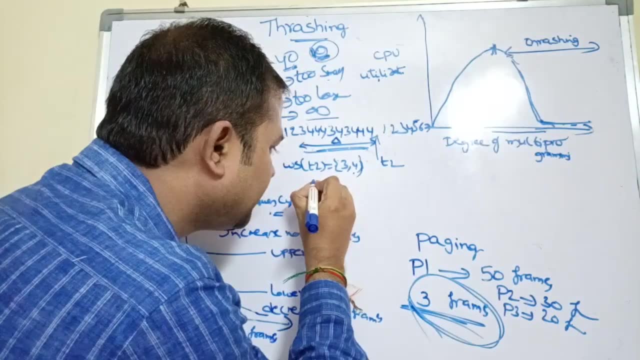 So only Two frames will be needed. So only two frames will be allocated for this working set. So here how the working set will work. is it works based upon the Suppose this is nothing but D? If D is less than M, 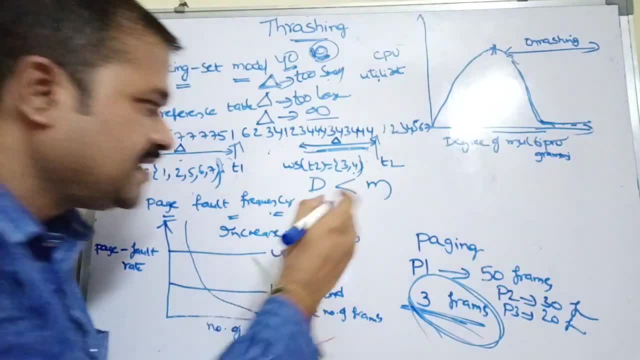 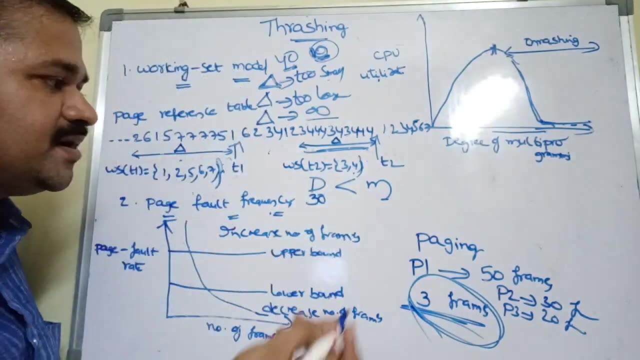 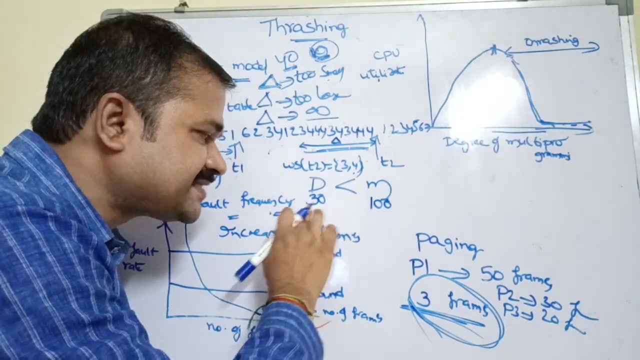 D stands for demand for the process, Whereas M stands for main memory frames. Let the demand for the process are 30. Whereas let us assume that main memory contains 100 frames. So what is the demand? The demand for our process: the process needs 30 frames for its execution, whereas main memory contains 100 frames. 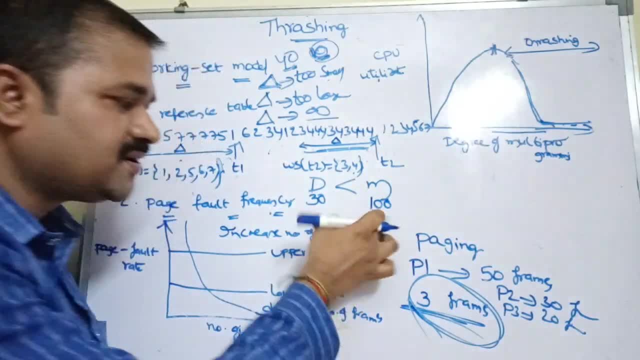 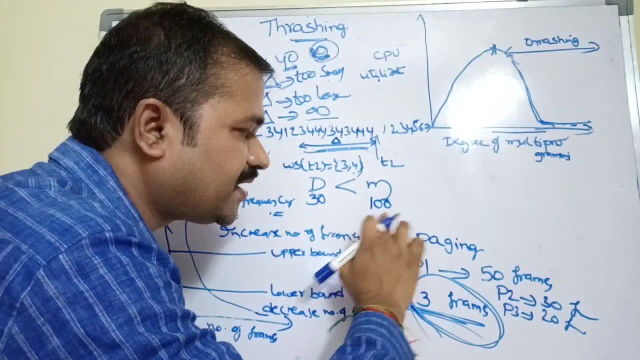 So here there is no problem. here 30 is less than 100. So we can. operating system can accommodate some more processes in the main memory. Why? Because 70 more frames are free now in order to utilize the CPU performance in an effective manner. 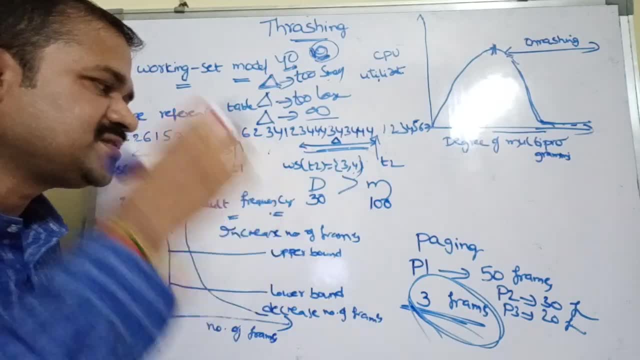 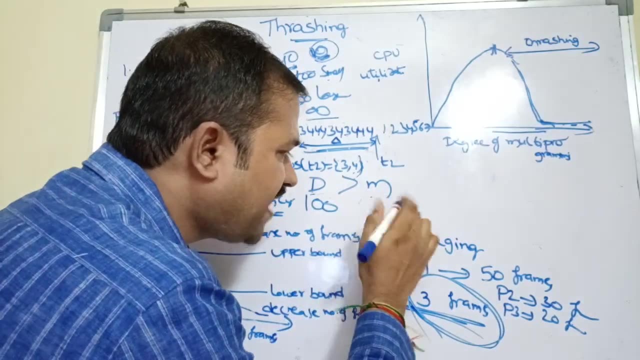 But let us assume that what happens if the demand of the process is greater than the size of the main memory? Let us assume that Demand of the process is greater than the size of the main memory. Demand of the process is 100. Whereas we have only 10 frames in the main memory. 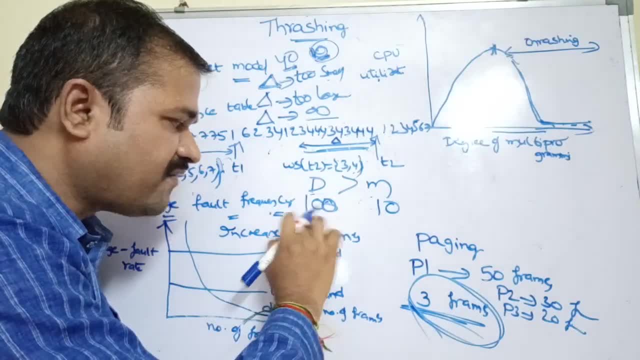 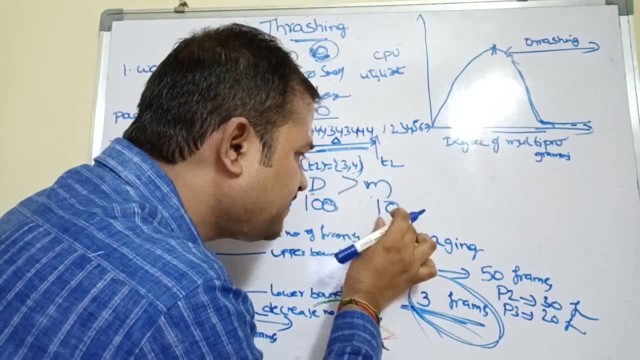 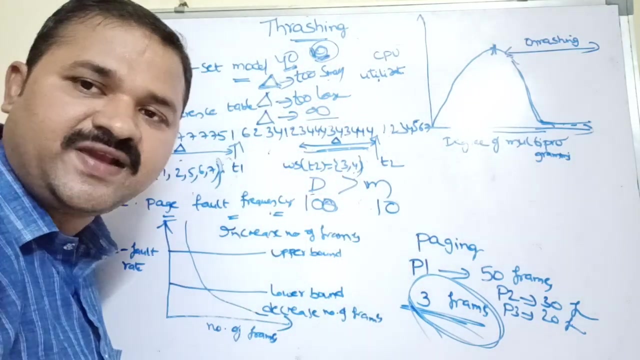 So what is the demand of the process? Our process requires 100 frames in order to complete its execution, Whereas what are the free frames in the main memory? Only 10 frames. So whenever the demand is greater than the available main memory frames, then trashing will occurs. 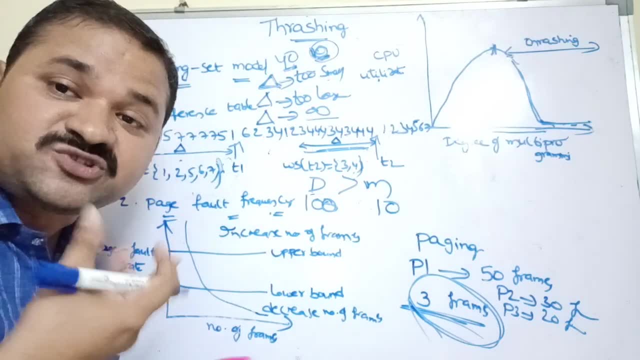 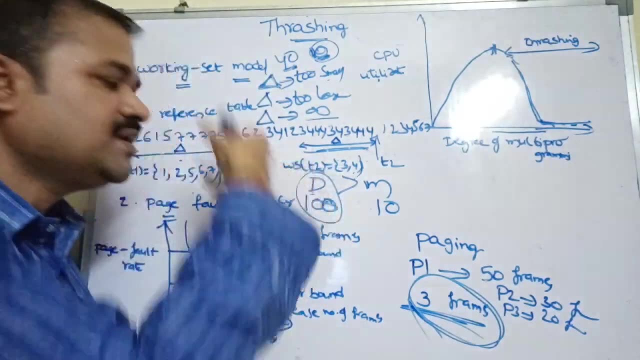 So whenever trashing occurs, then operating system has to suspend one of the process in the main memory And allocate, And allocate the suspended process frames to some other process- Trashing. So this is the first approach. Let us see the second approach. 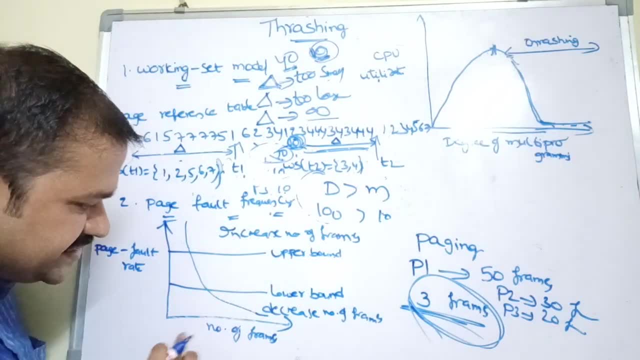 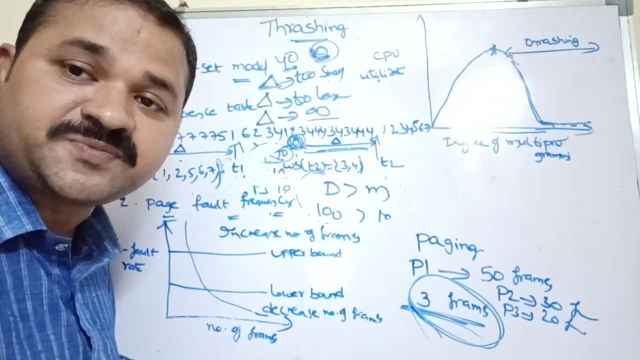 The second approach is phase fault frequency. Here the x-axis represents the number of frames, Whereas the y-axis represents phase fault rate. We know that trashing occurs mainly because of higher number of phase faults, So we have to control the phase fault.